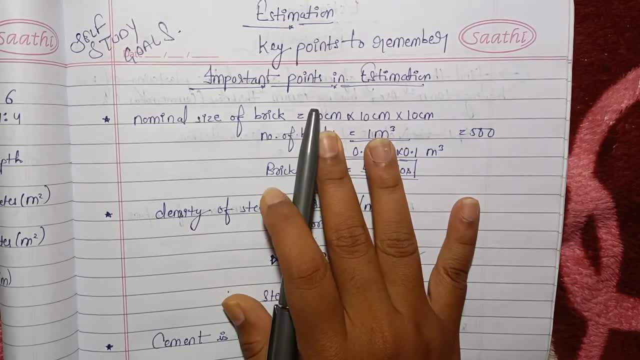 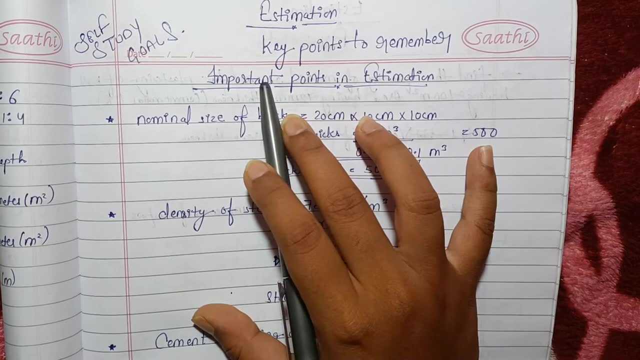 Hello everyone, welcome back to my YouTube channel. From this video we are going to start our new series, that is estimation Okay. so before starting the estimation series, we will discuss some key points that are important before starting the estimation series: Okay. 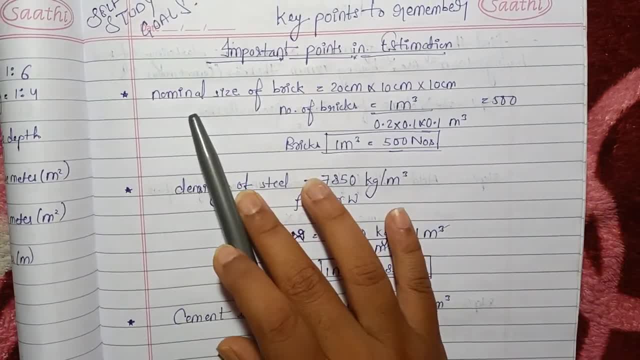 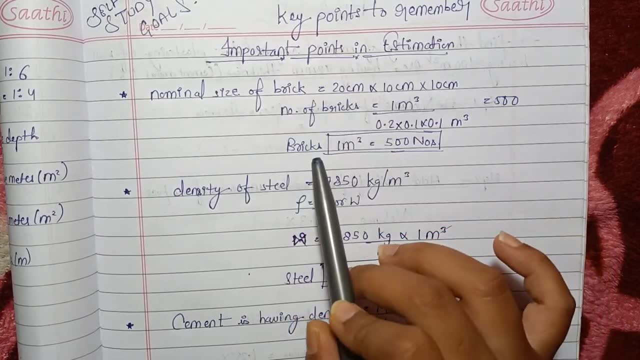 so we will see all the points one by one. First point is that the nominal size of a brick. Okay, so you have to know the nominal size of a brick, because if you find the number of brick required for a particular area, then you have to know the nominal size of. 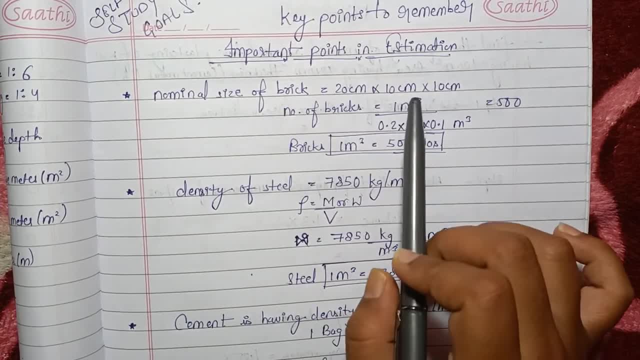 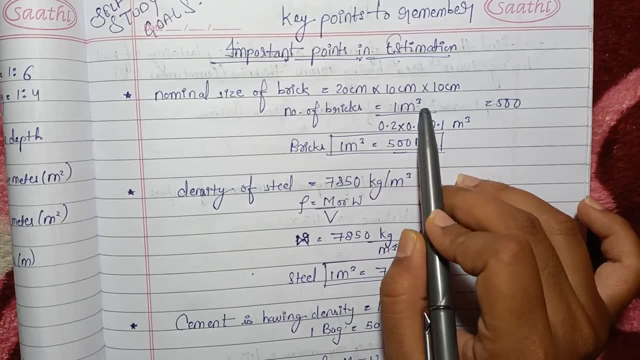 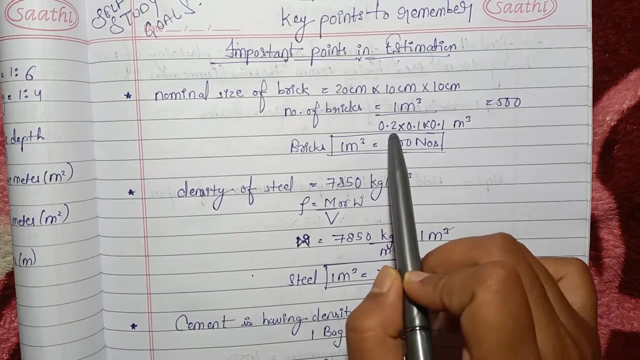 a brick. So nominal size of brick is 20 cm by 10 cm by 10 cm. Okay, to find the number of brick, what formula will you use? Assume that you have to find out how many bricks are used in 1 cubic meter. Okay, so you will divide 1 cubic meter by its nominal size: Nominal. 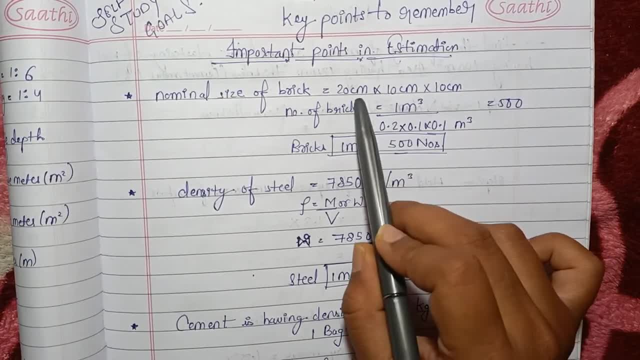 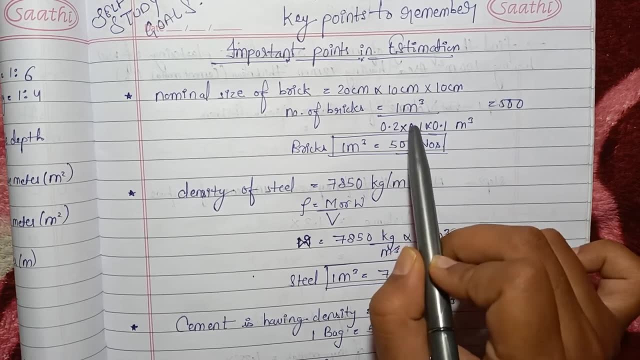 size will be converted into meter, so it will be 0.2, 20 cm and 10 cm will be 0.1.. Then again it will be 0.1 meter. So meter, meter, meter, meter. cube will be free. So when? 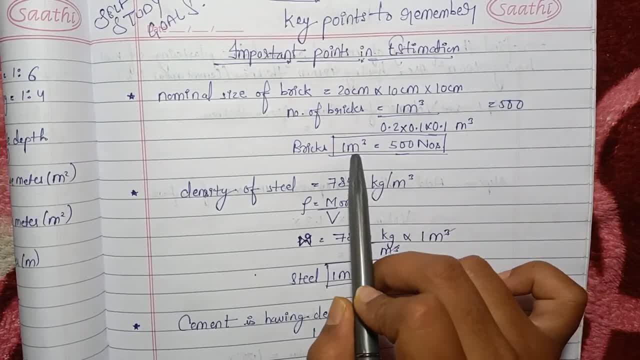 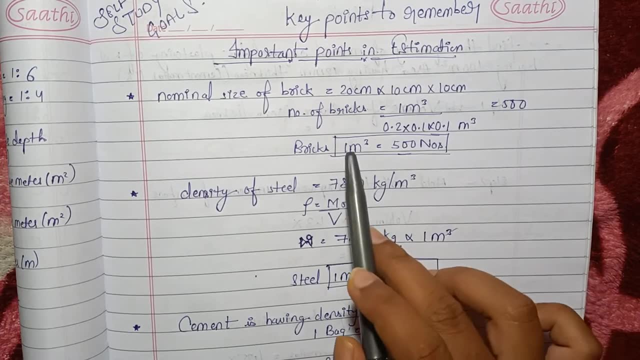 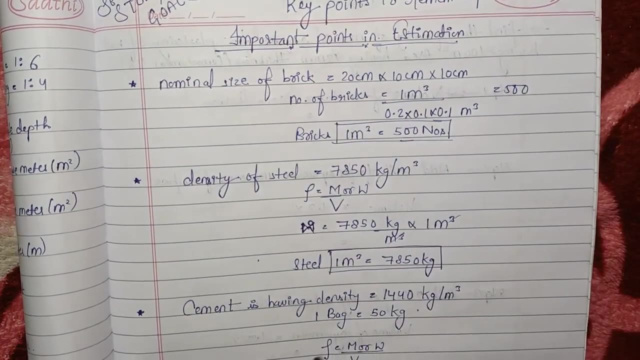 you divide it, then yours will be 500. Okay. so what did it mean? you can say here that 500 number of bricks are used here in 1 cubic meter. Okay. so in 1 cubic meter, 500 number of bricks are used. Okay. so this is the first point. You should keep this thing in mind. 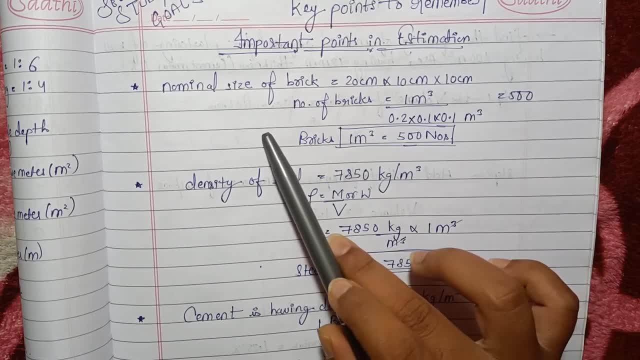 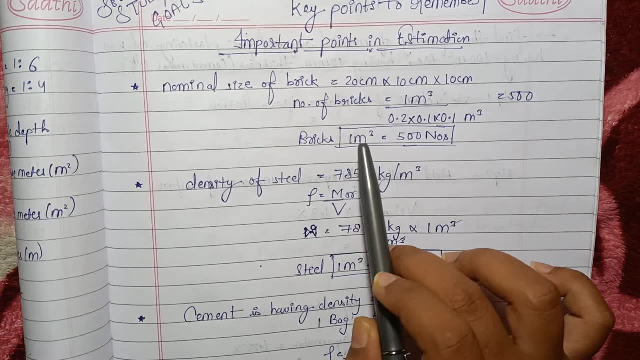 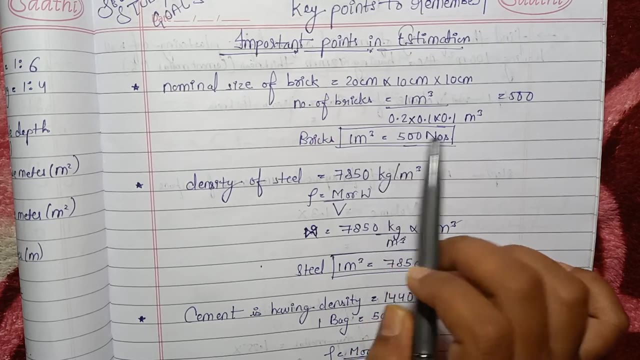 because sometimes direct questions are asked, For example how much brick you have to use in 5 cubic meter. So you can directly multiply there. if you know that, how much brick you have to use in 1 cubic meter, If 500 is used in 1, then you can take out in 5 or 10 by simply multiplying. 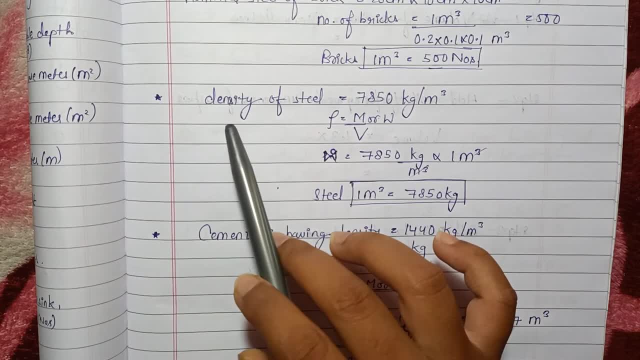 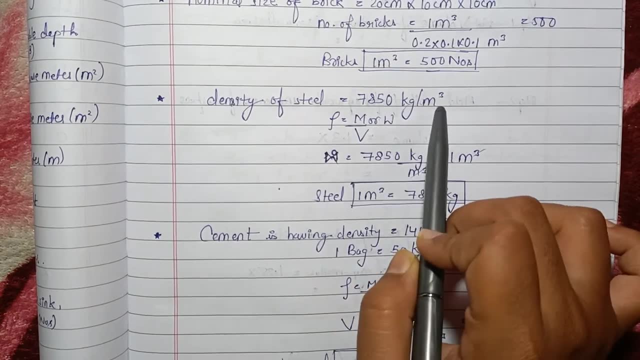 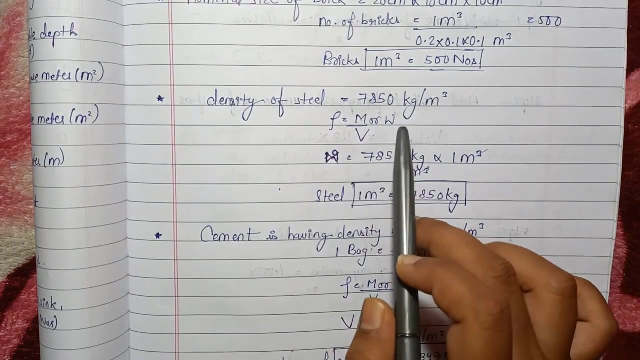 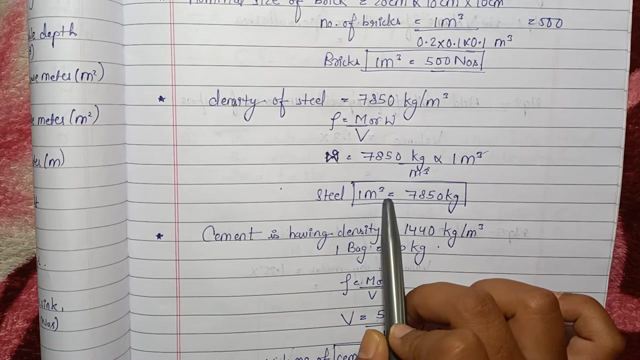 Next we will see the second point. Second point is the density of steel. You know the density of steel is 7850 kg per meter cube. The density of steel is 7850 kg per meter cube. If you know the density of steel then you can take out how much steel is used per meter cube. 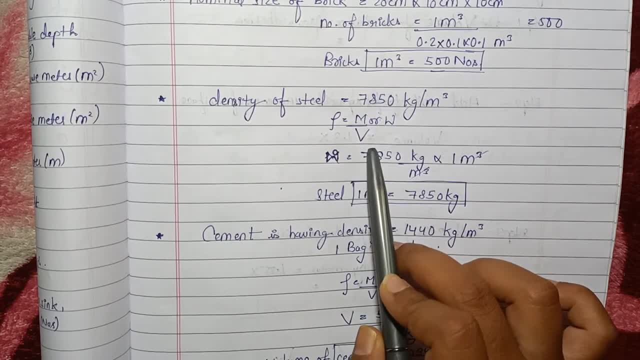 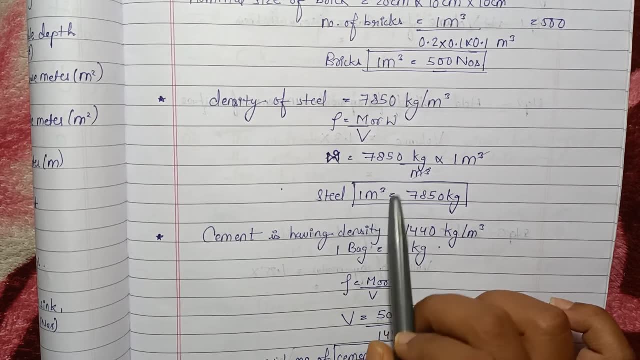 Density equals to mass upon volume, or you can say weight upon volume. So you have to take out the weight here, that how much weight is used per cubic meter. If you take out weight then it will be density into volume. So you know the density. 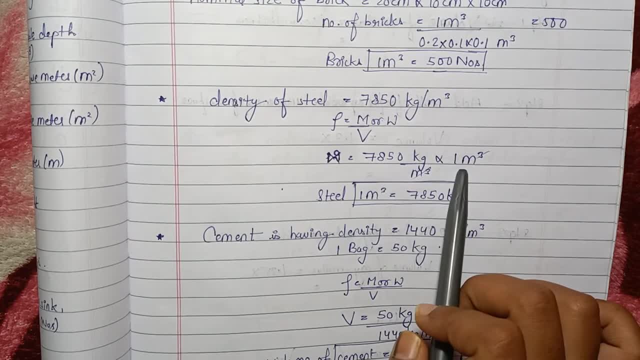 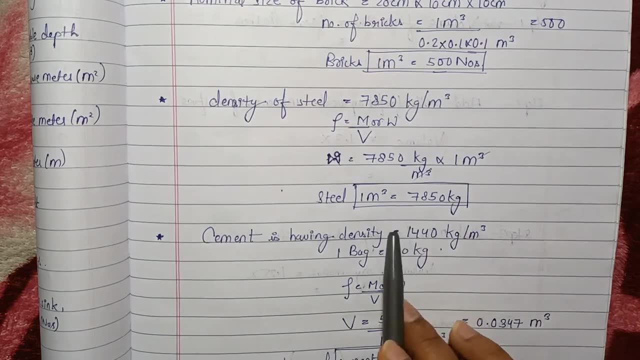 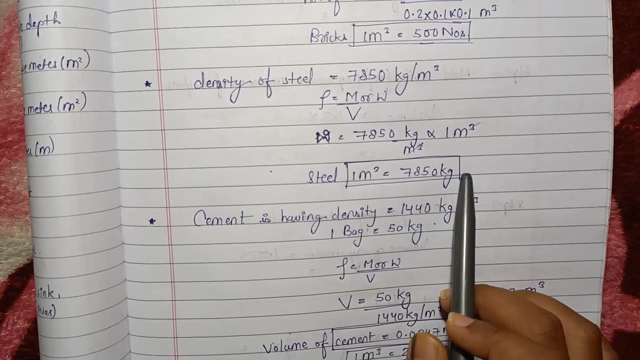 So your density is 7850 kg per meter cube And the volume you are taking out for which? For 1 cubic meter. So if you multiply 1 cubic meter, then cubic meter and cubic meter will be cancelled And your 7, 850 kg is used in 1 cubic meter. 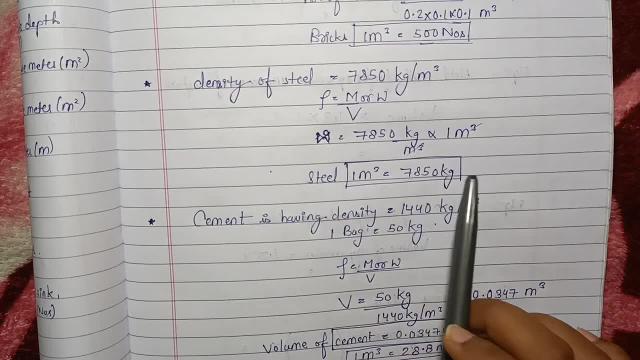 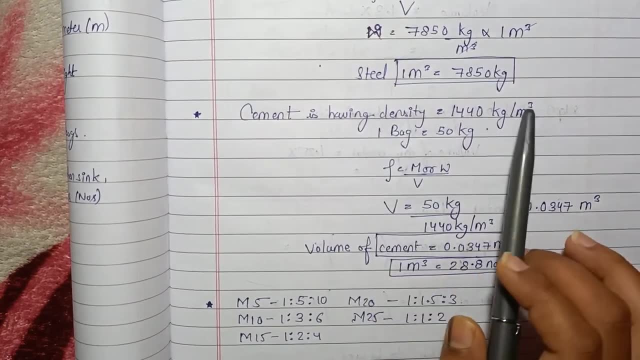 7, 850 kg of steel is required in 1 cubic meter. Next we will see third point, that is, cement. Cement is having a density of density of 1440 kg per meter cube. one thousand four hundred forty kg per meter. 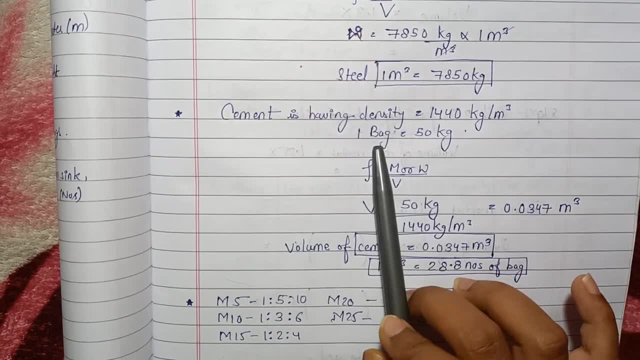 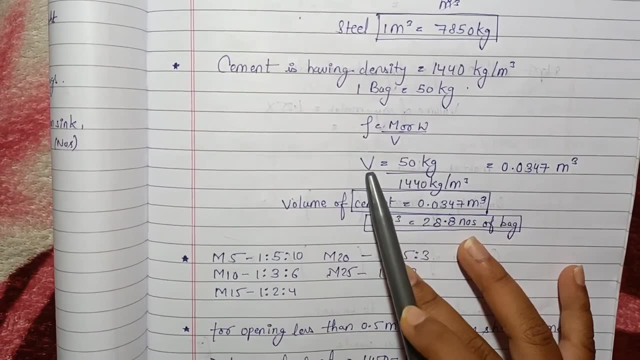 cube egg bag meh 50 kg ka bag hota hai. generally egg bag jo hota hai 50 kg ka hota hai. toh yaha par aap density equals to weight upon volume kar rahe ho, aur aapko yaha par volume nikalna hai, volume, kitna volume of cement hota hai, aapka, toh vo kya. 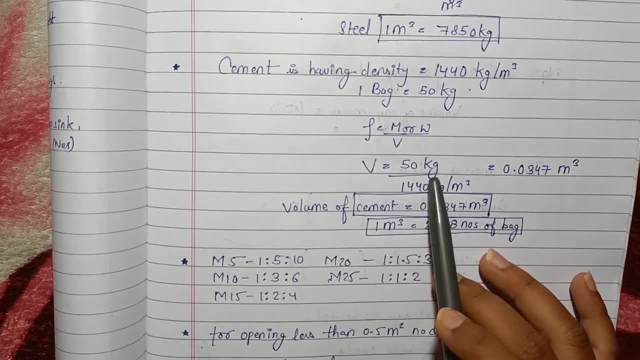 ho jayega volume yaha rahe jayega aapka yeh kya ho jayega? weight upon density: weight kitna hai aapka 50 kg egg bag ke liye? aur density of cement: aapko bataya abhi 1440 hota. 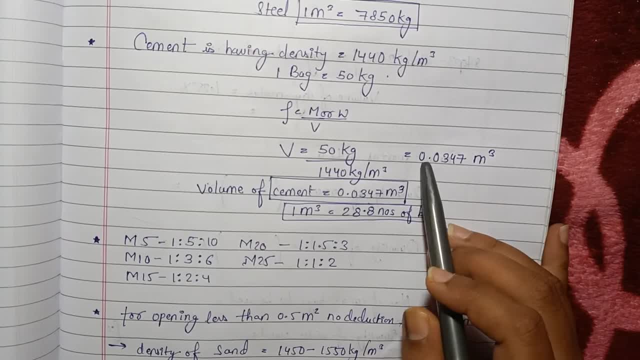 hai toh weight upon density. aap karoge, toh aapka volume of cement aajayega tike kais sari jagay meh aapko diya rata hai. volume of cement will be equals to 0.0347 meter cube. 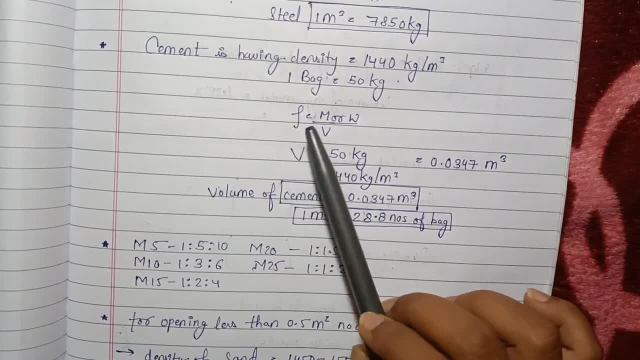 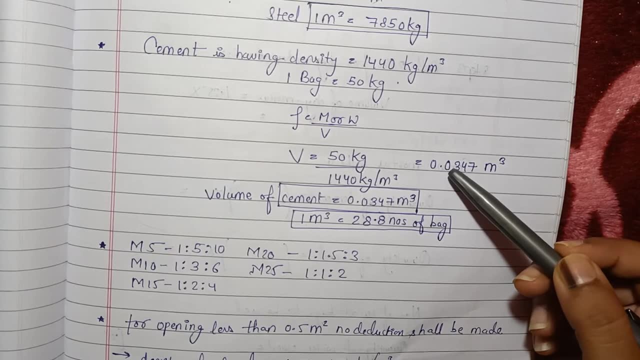 yeh aaya, kaise yeh maine aapko yaha par bataya tike simple density, mass aur volume ke relation. se aap nikal sakte ho tike, agar aapko yaha par kabhi kabhi confusion ho jata hai, ki 0.347. 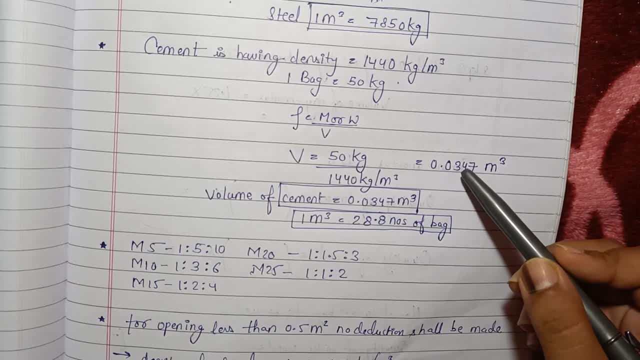 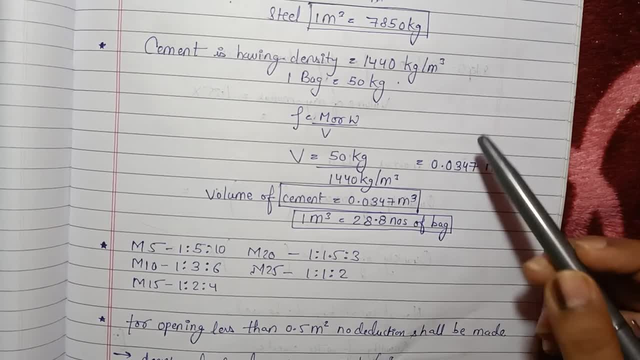 jab aap solve karte ho, numerical usr time, kabhi kabhi confusion ho jata hai, toh iss se better hai. aaya kais yeh aap bhi jaan lilijeya, that ki aapko yaad na karna padese, So volume. 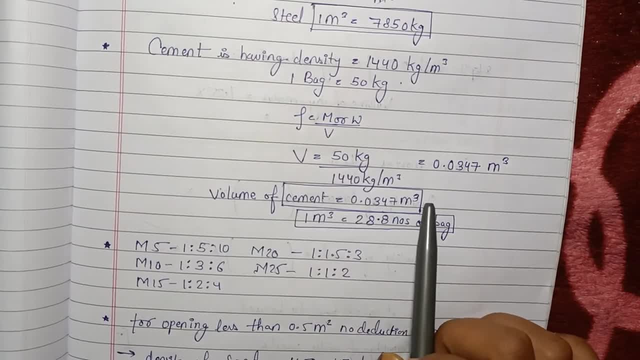 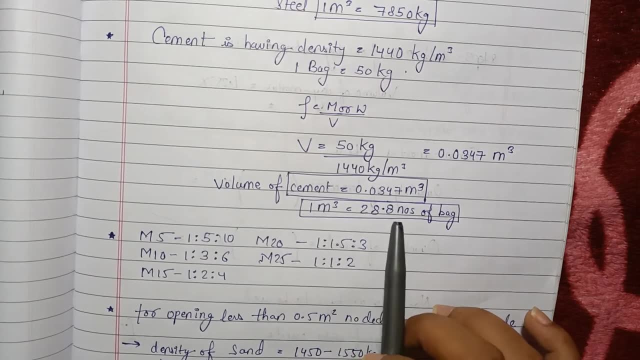 of cement will be equals to 0.0347 cubic meter. So ameter cube mein aapke kitne number of bags used hota hai. A meter cube man aapke 28.8 number of bag used hota hai, yeh bhi aapko. 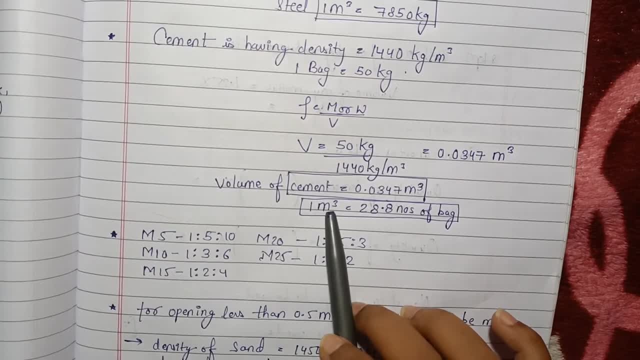 dhiaan marknaya balance. hain reo karo大家都аф hisce you have put. Hallo, If surface volume of all cements are in meter cube, get a difference in cements. hain main 我是 do ksi crack. 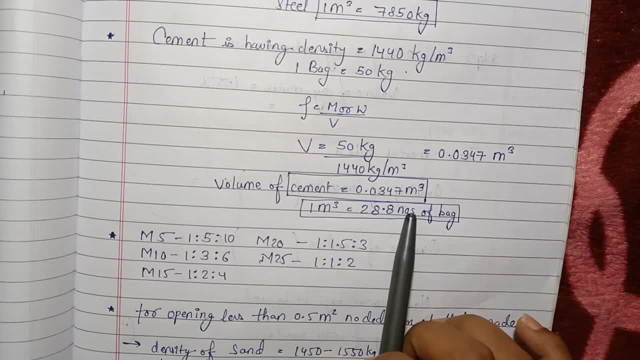 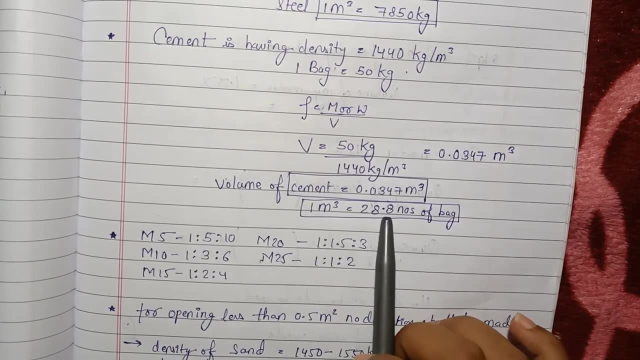 you have to calculate the number of bags as well, Because you cannot purchase in meter cube, So you have to purchase in number of bags. So if you need 28.8 number of bags in 1 meter cube, then you can calculate the number of bags in 2 meter cube. 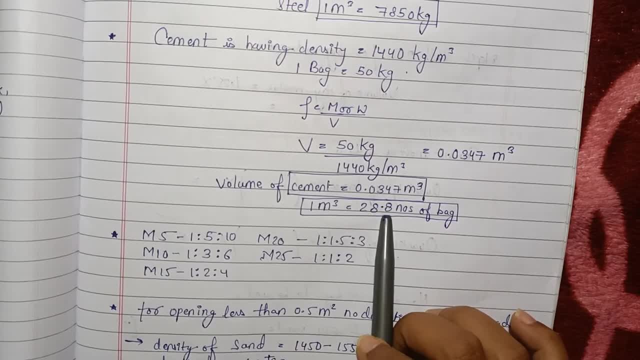 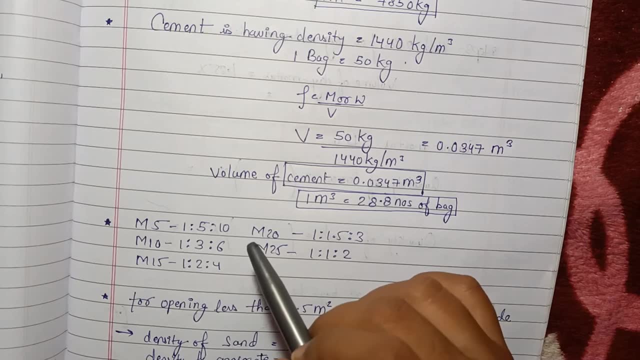 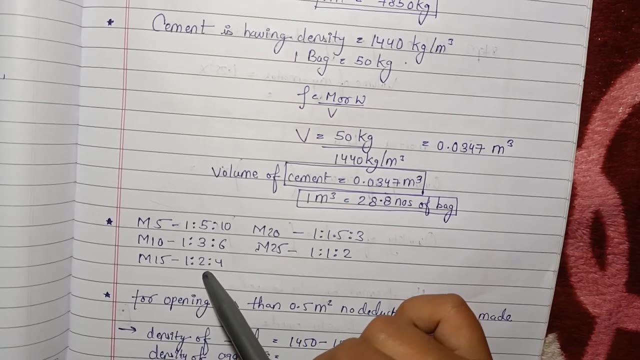 or 10 meter cube by simply multiplying them. Okay, Now let us see the next important point in estimation. When we solve the question of estimation, then we need its ratio. These ratios are very important. We read this in RCC also. 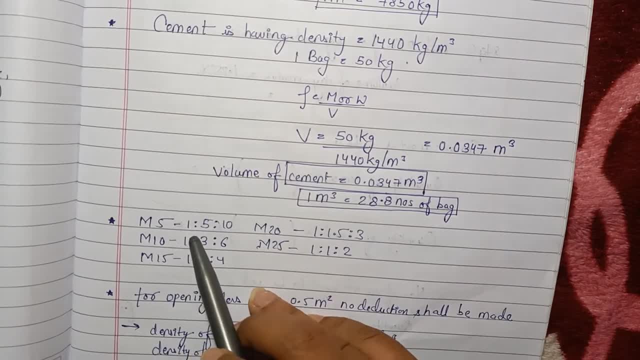 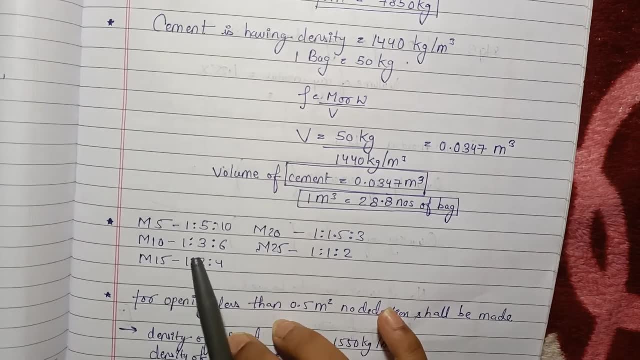 These are general basics, Everyone should know, But we will revise it once again before starting our estimation series. So M5's ratio is 1 is to 5 is to 10.. M10's ratio is 1 is to 3 is to 6.. 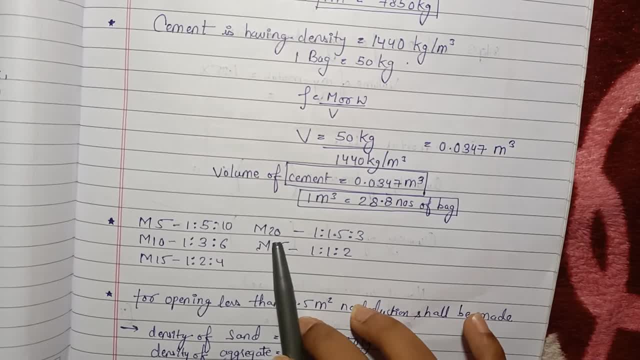 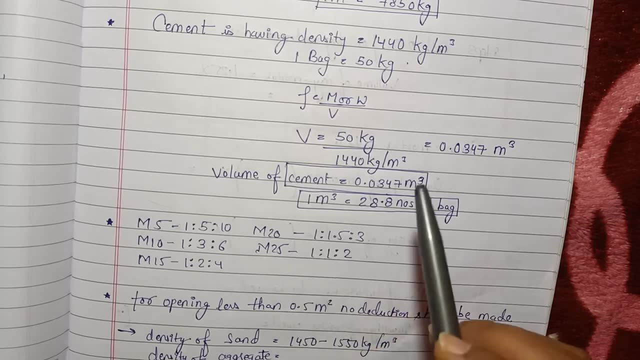 M15's ratio is 1 is to 2 is to 4.. M20's ratio is 1 is to 1.5 is to 3.. M25's ratio is 1 is to 1 is to 2.. Okay, 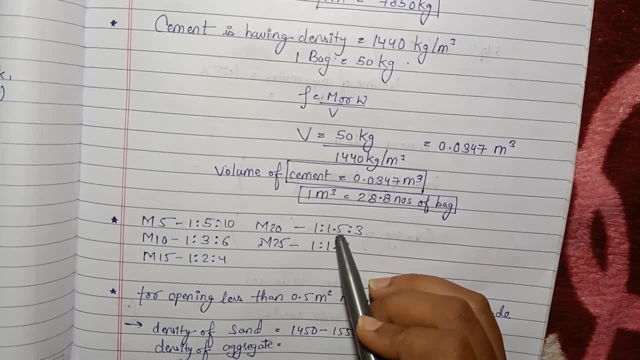 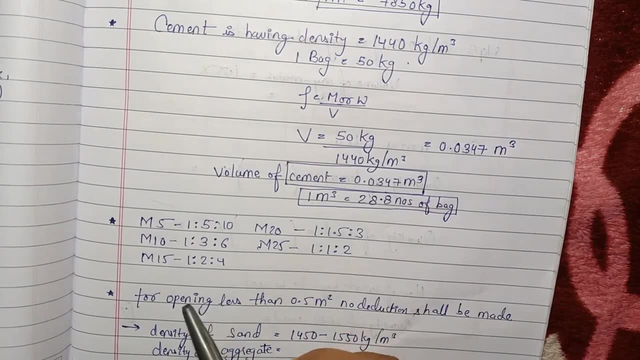 You have to keep in mind that M20's ratio is: 1 is to 1.5 is to 3.. Okay, Here, 1.5 is there and 1.5 is doubled to 3.. You have to keep this in mind. 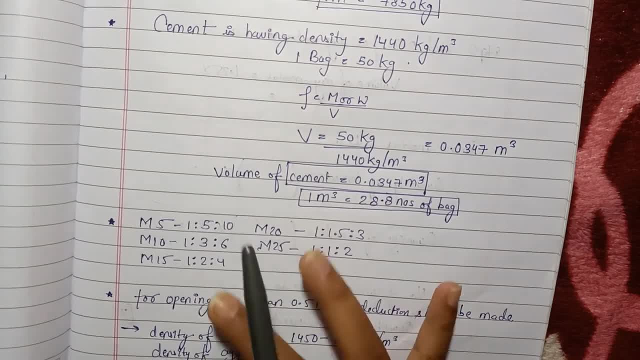 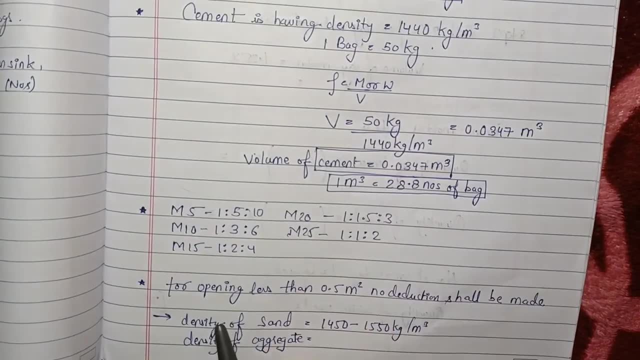 And you should also keep in mind M15's ratio: 1 is to 2 is to 4.. You should generally keep these two in mind. Next we will see some important points which you should know For opening less than 0.5 square meter cube. 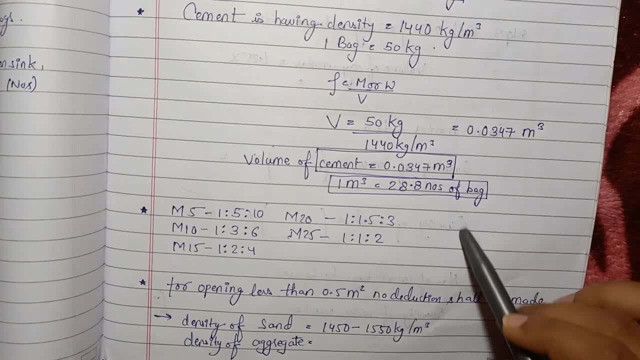 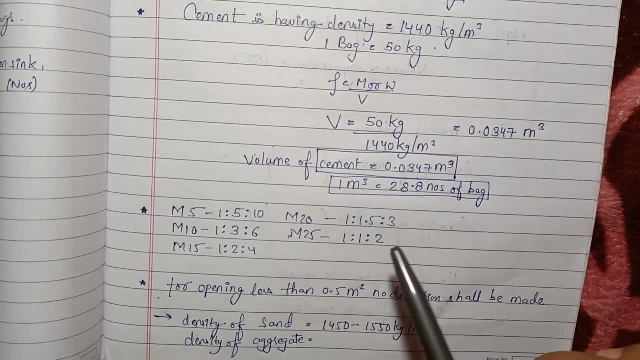 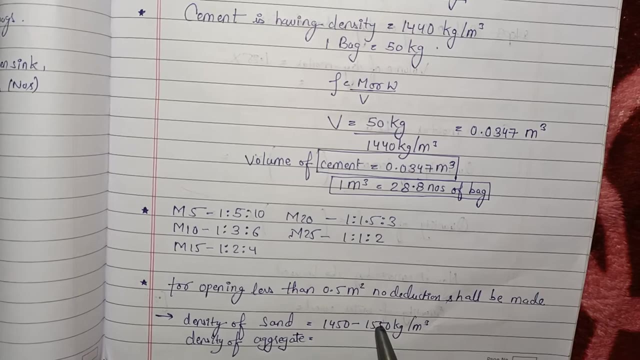 no deduction shall be made. If you have a wall with 0.5 square meter opening, then you should not take deduction there. If you have a wall with 0.5 square meter opening, then you should not take deduction there. Density of sand is from 1450 to 1550 kg per meter cube. 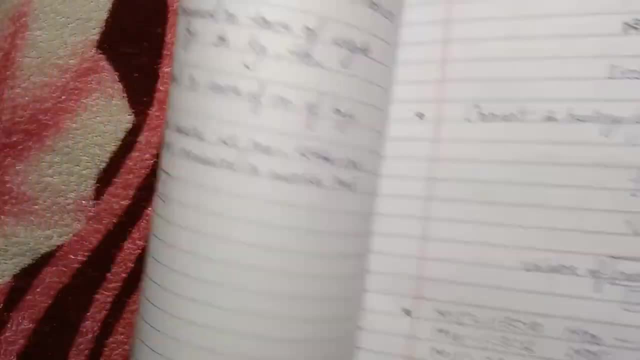 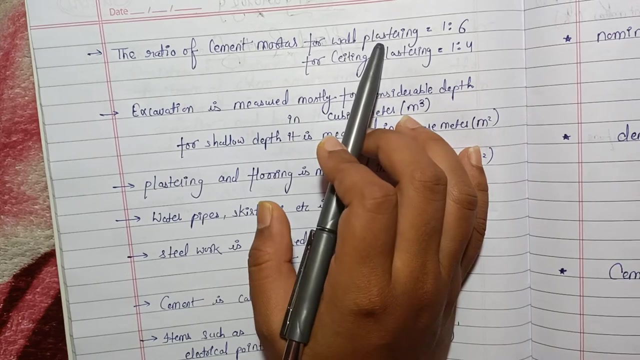 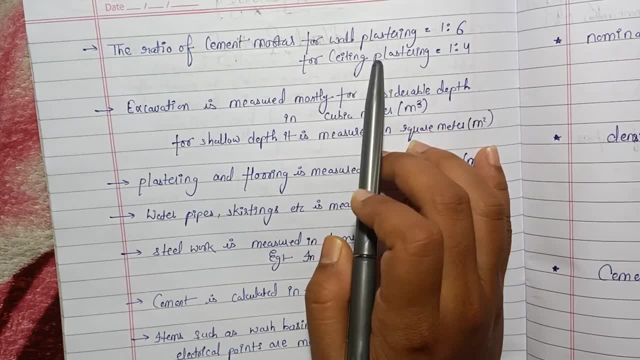 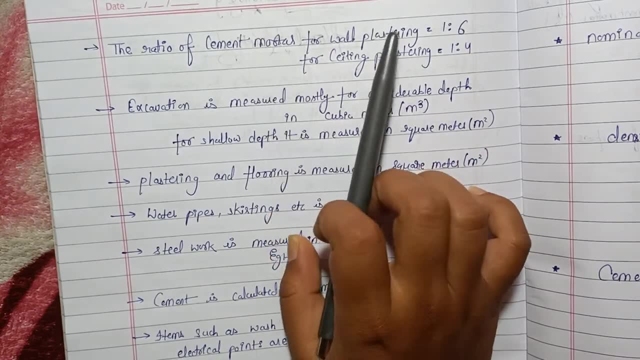 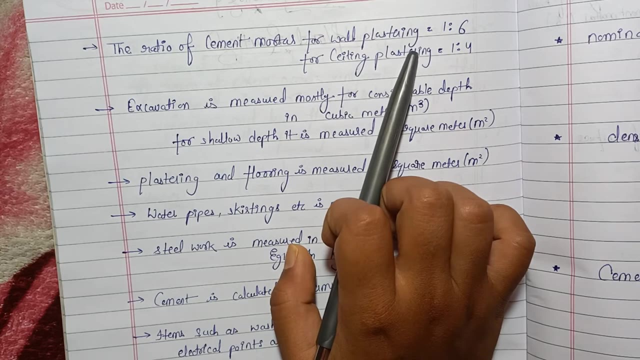 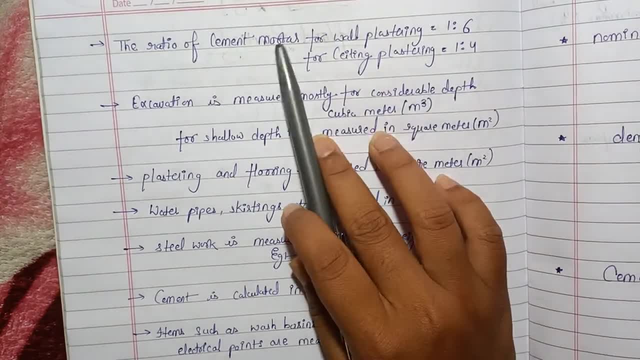 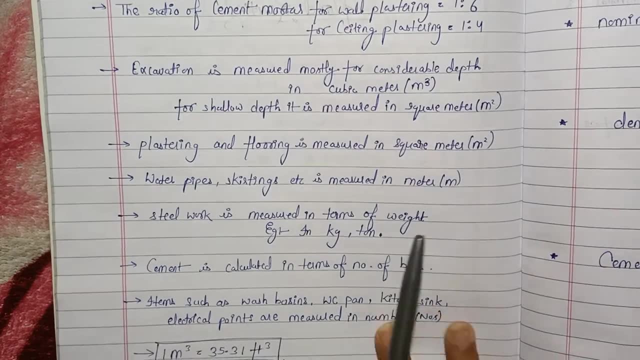 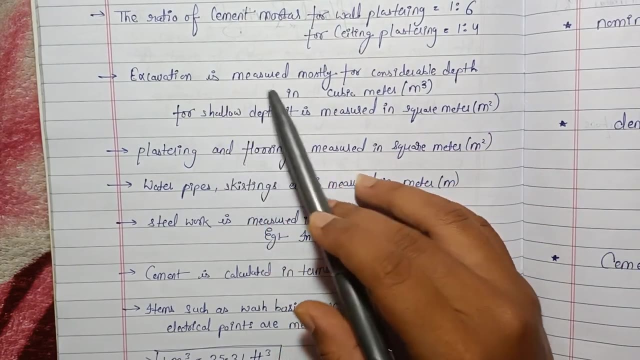 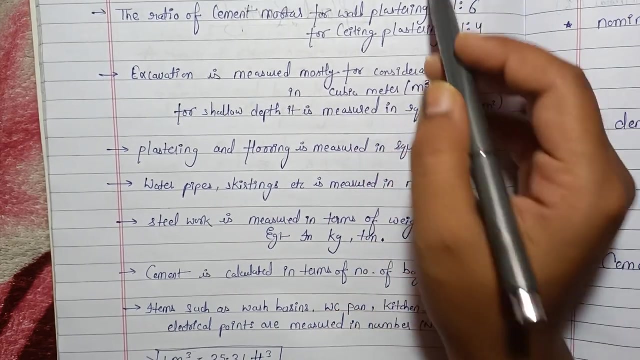 The ratio of cement mortar for wall plastering. The ratio of cement mortar for ceiling plastering. The ratio of cement mortar for skin plastering. The ratio of cement mortar forsite plastering. The ratio of cement mortar for καιap plastering. 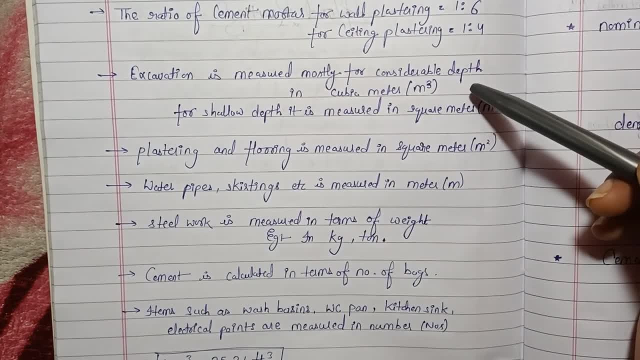 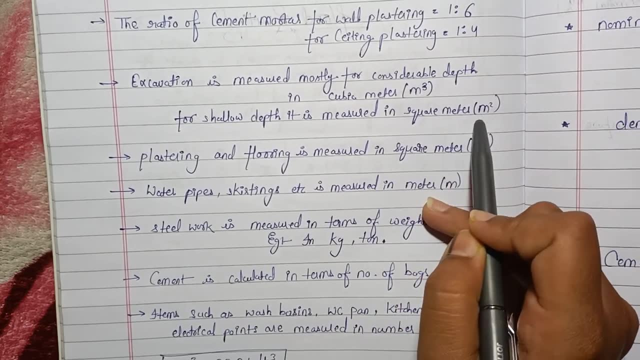 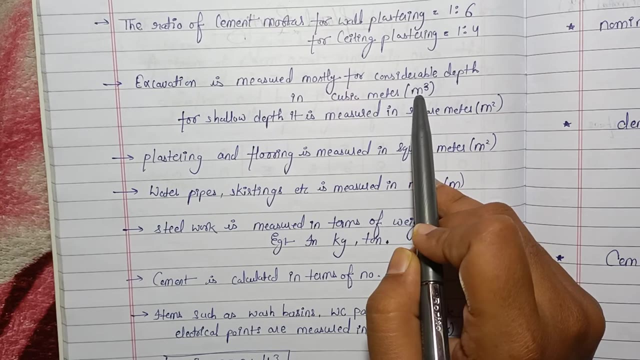 But if you are doing an excavation for something else, for example, whose depth is not very considerable, it is very low, then in that case only you will take the excavation in square meter, that is, in meter square. Generally, when we do an excavation whose depth is more, we take it in cubic meter only. 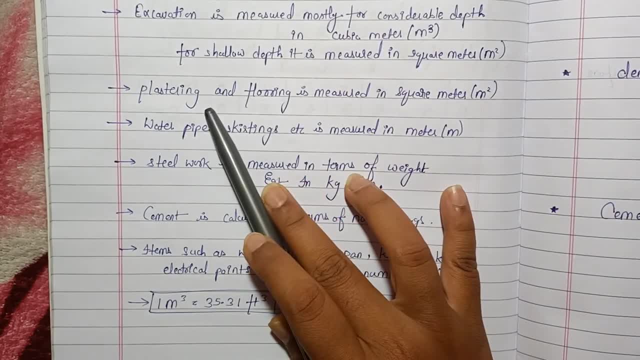 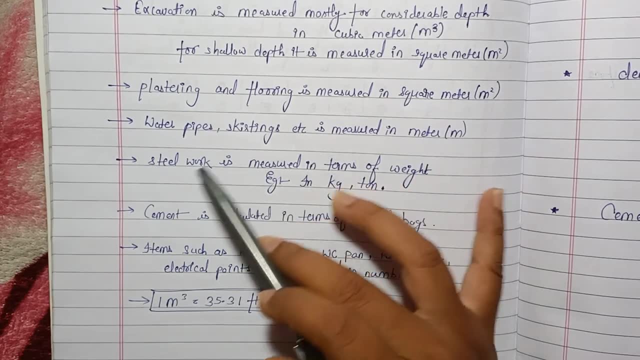 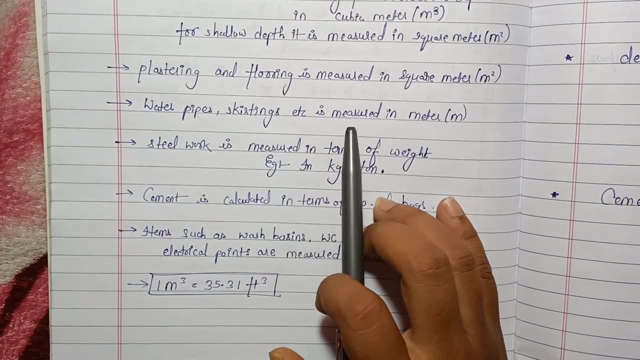 When you do flooring and plastering. in the case of flooring and plastering, there is always a measurement in meter square. When you give a contract to a contractor, then they measure it in meter square In. what are water pipes and skirting measured In meter? 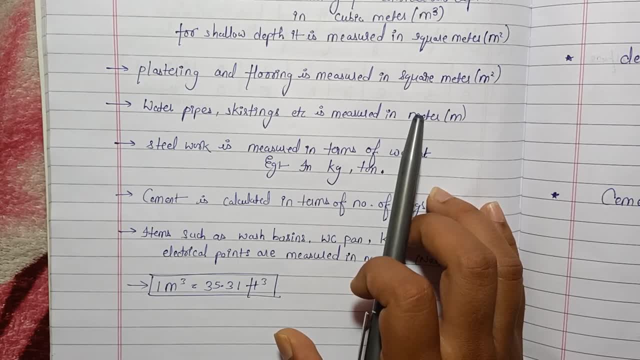 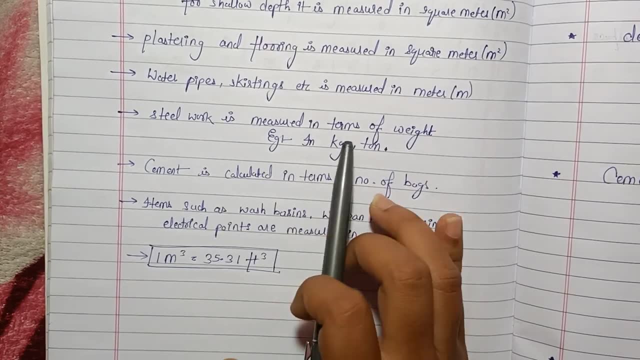 If you buy water pipe and skirting or give it in contract for work, then it is purchased in meter and goes in contract in meter. Steel work is measured in terms of weight. Steel is measured in terms of weight Generally. it is not measured in cubic meter. 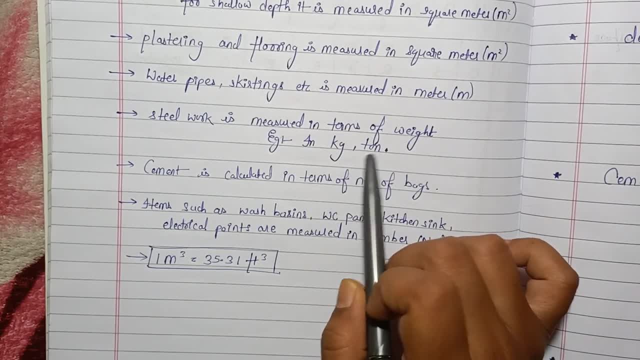 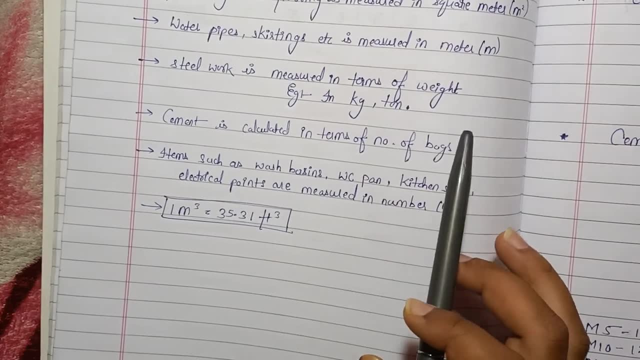 It is always measured in terms of weight. Weight is measured in terms of kg. ton quintal Cement is calculated in terms of number of bag. I had told you that if you calculate the quantity of cement then it will come in cubic meter. then you have to convert it to number of bag.